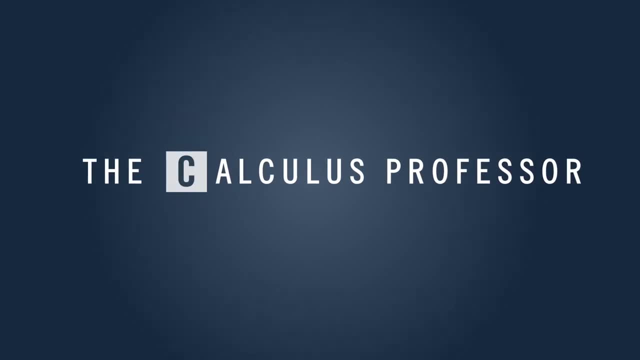 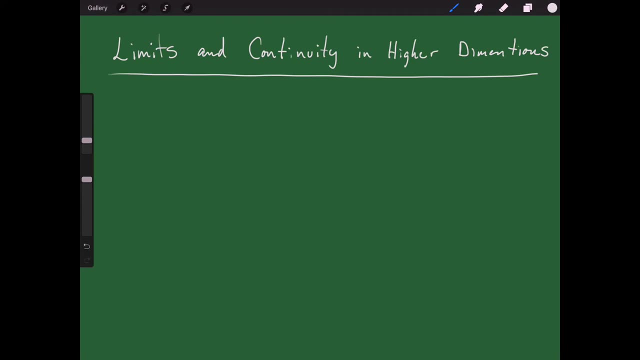 Welcome back. Today I'd like to talk a little bit about limits and continuity and higher dimensions. So I want to start with a definition. So definition: we say that a function f of x, y approaches the limit, L as the point approaches some specific point- x sub 0,, y sub 0, and write. 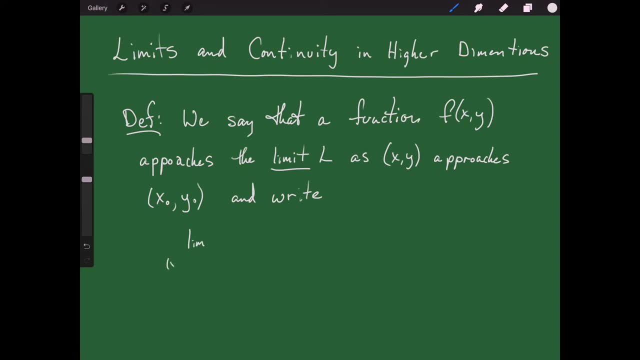 that the limit as x- y approaches x sub 0, y sub 0 of f of x- y equals L if for every number epsilon that's bigger than 0, there exists a number delta greater than 0 such that um. 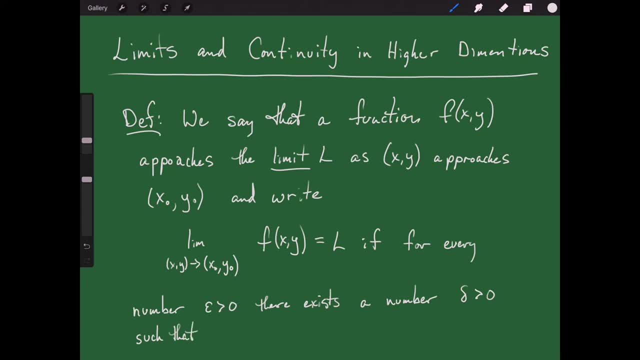 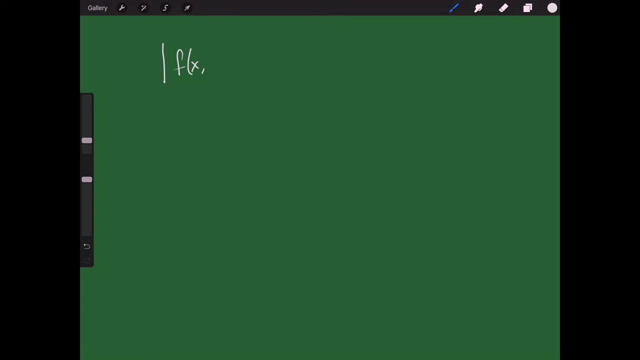 um, um, um for all. a minus L is less than epsilon whenever 0 is less than the square root of x minus x0 squared, plus y minus y0 squared is less than delta. Okay, so you can look back over that definition a couple times if you need to. 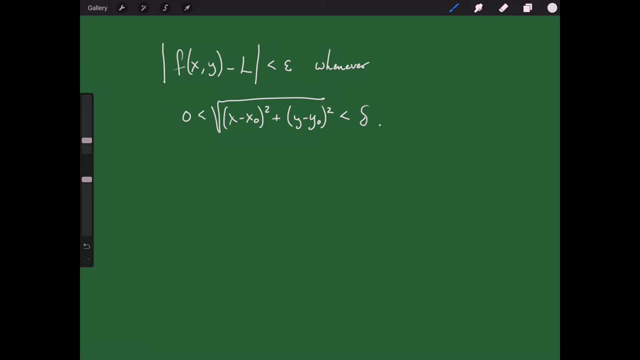 but it's saying something sort of simple and that is, what does it mean for the distance between xy and x0, y0 to get to the square root of x, To get close together? If it's close together, then this number is getting small. 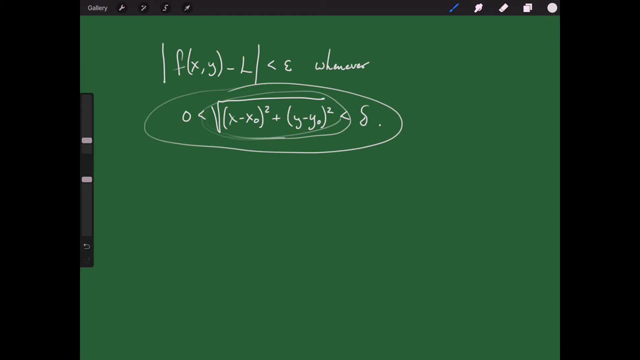 And it's saying that if you get this number small enough, in other words, if you get the point xy and x0, y0 close enough to each other. so let's say we have a point here, xy and we have another point here. let's call this x0, y0,. 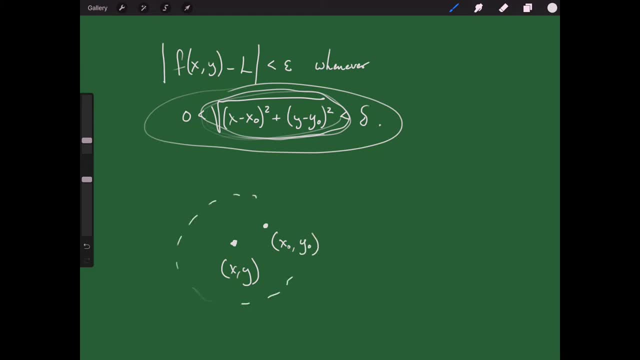 and let's say that we have a point here xy, and let's say that we have a point here x0, y0, and we know that those two points, this is a circle around xy, and I know that that, let's say, has radius delta. 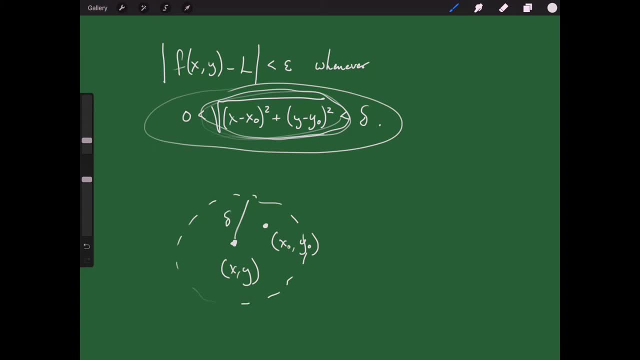 Okay. so if I know that this point x0, y0 is within delta of xy, then I'm guaranteed that the function is close to the limit value. In other words, the functional value of of this point xy is close to L. 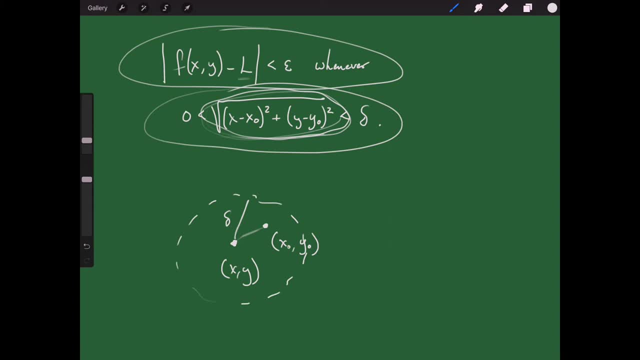 This is exactly the same as what our limit is in two dimensions, but now we're dealing with an extra dimension that this original point can live in. So if we know that x0, y0 is close to xy, then we know that also the functional value is getting close to the limit value. 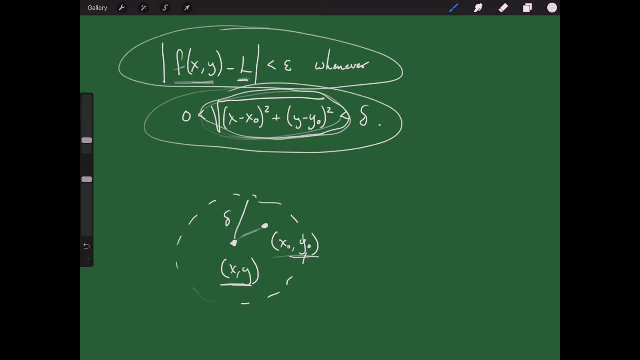 And that's what we say. it means for a function to have a limit L. Okay, now that we know that, let's talk about some of the properties of limits when we're dealing with an extra dimension. So this is a theorem: Properties of limits. 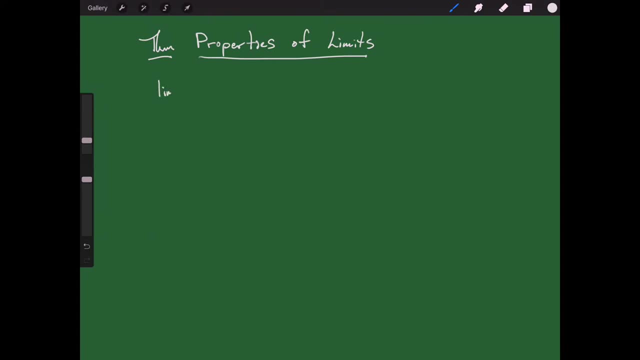 And we're going to start with the limit as xy approaches x0, y0 of f of xy, Let's call this capital M, And the limit as xy approaches x0, y0. Of f of xy, Let's call that L. 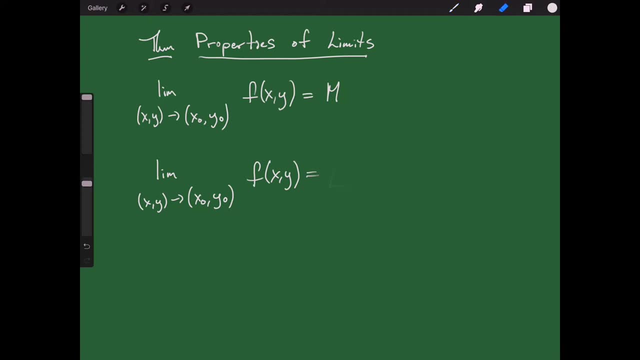 Oh, I'm sorry, I made a mistake here. Let me rewrite: Of g, of x, y, Let's call that L. Okay, so then we get some properties, And the first property that we have is: what, if we're taking the limit? 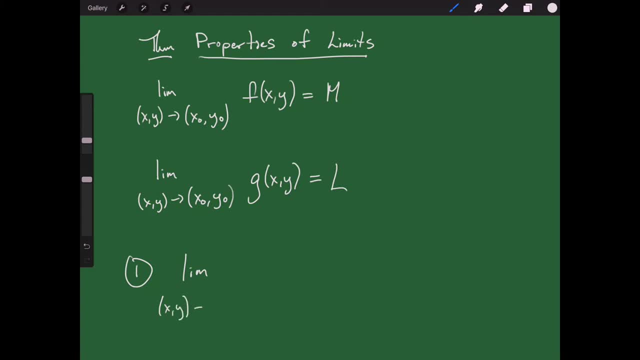 as xy approaches x0, y0 of f of xy plus g of xy. Well, it looks exactly like limits do in two dimensions. We can just distribute that limit across this sum and take the limit of each one individually, And then we get M plus L. 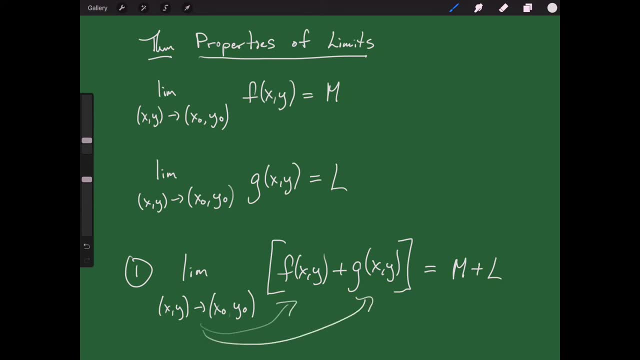 So that limit can distribute across a sum: Okay. second property that we get is that the limit as xy approaches x0, y0 of f of xy- Okay. second property that we get is that the limit as xy approaches x0, y0 of f of xy. 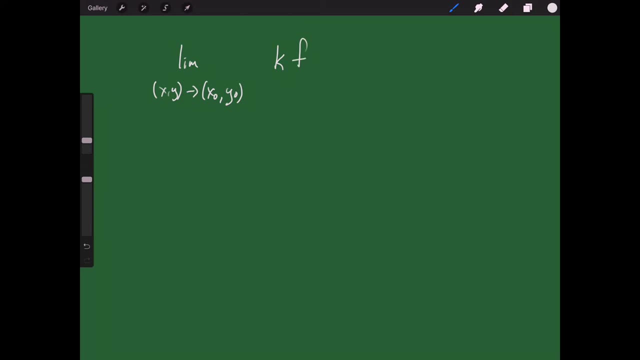 Soonst of K. a constant times f of xy is equal to K times M. In other words, this constant K can move outside of the limit if we would like first, And then we just take the limit of f of xy, which is M. 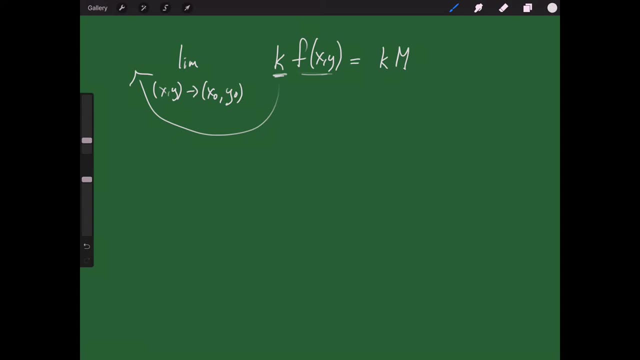 so constants can move in and outside of limits with no problems, just like they always have been able to do. Okay, we also get that the limit as x y approaches x0, y0 of f of x y, g of x- y is equal to m times l. 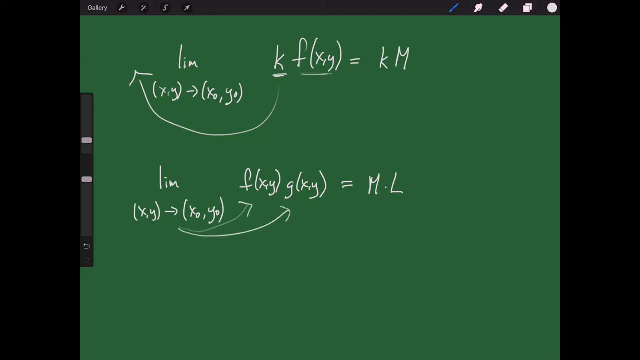 In other words, a limit can be distributed over a product of functions. We get that the limit as x y goes to x0, y0 of f of x y divided by g of x y, then this is going to be equal to m divided by l. 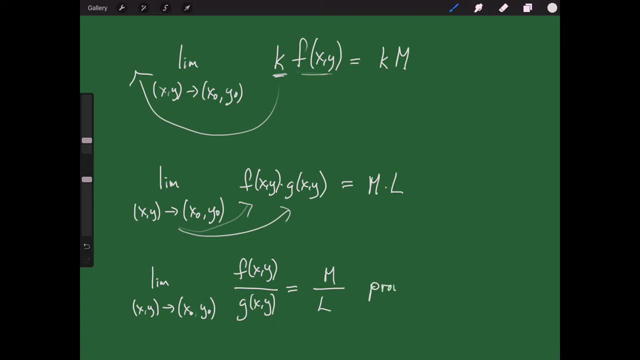 provided m divided by g of x y, that l is not 0.. Okay, and finally one more. We get that the limit as x y approaches x0, y0 of f of x y to some power. Let's say: 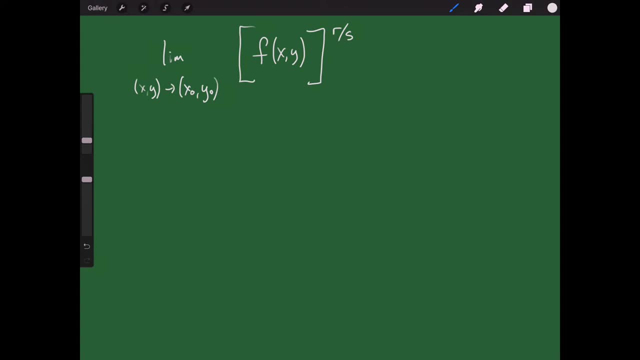 that we raise it to the r over s power, Then this is just going to be m raised to the r over s power. Okay, so any fractional power that I raise that thing to the limit can just move inside the power, and I can take the limit first and then raise it to the power. 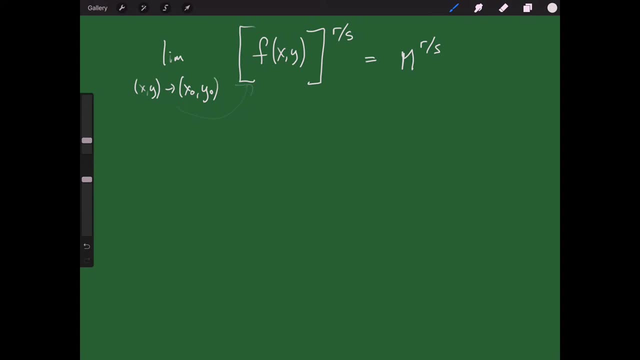 Okay, so basically all the rules that we already had for limits in two dimensions also apply to limits in three dimensions, and that's all we're really trying to say. So all the things we know about limits We can still use. Okay, let's do an example to kind of show how this works. 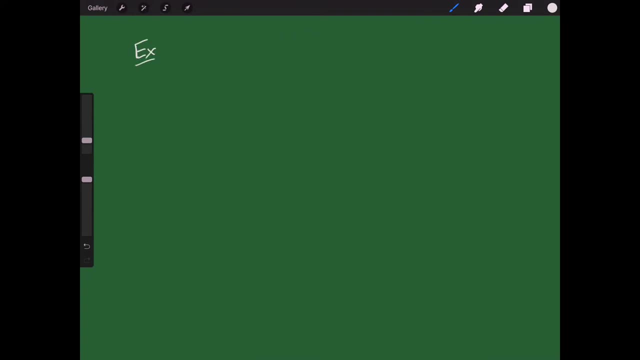 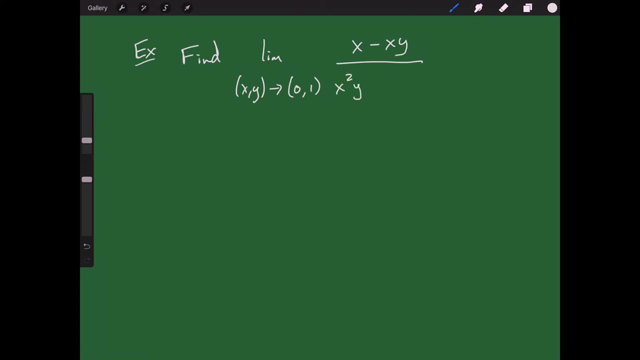 x squared y minus x minus y. Okay, so we've got to kind of go back to the basics and just remember, when we took limits to begin with, what was the very first thing we would always try, and that is: well, can I just plug in the point? and if I can just plug in 0, 1 and I don't get any division by 0, then we're done. 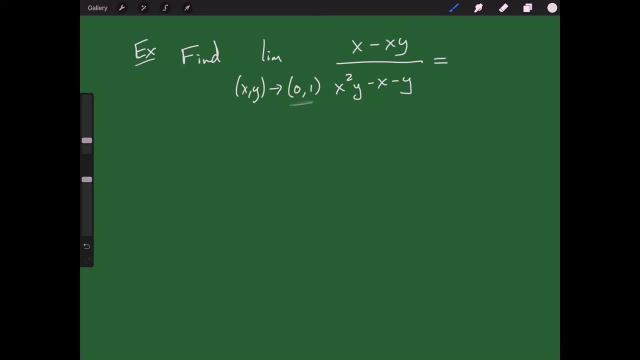 We get our limit, And so we should try that. So if I plug in 0 for x, notice the top just becomes 0. And on the bottom I get 0 minus 0 minus y. Well, y is 1, so I get minus 1,, which gives me 0. 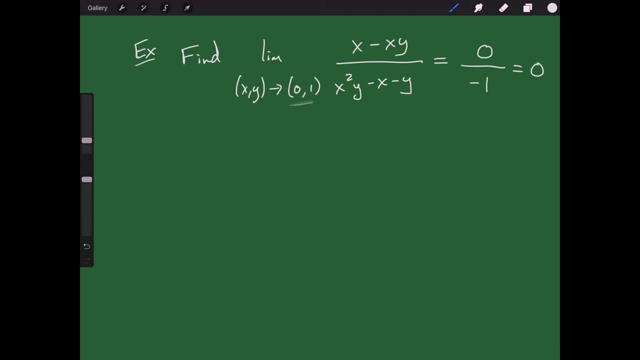 But 0 is not division by 0.. 0 is a number. That's perfectly fine. So I get my answer and my answer is 0.. Okay, let's do another example. Let's find the limit as x, y goes to a 3, 4 of the square root of x squared plus y squared. 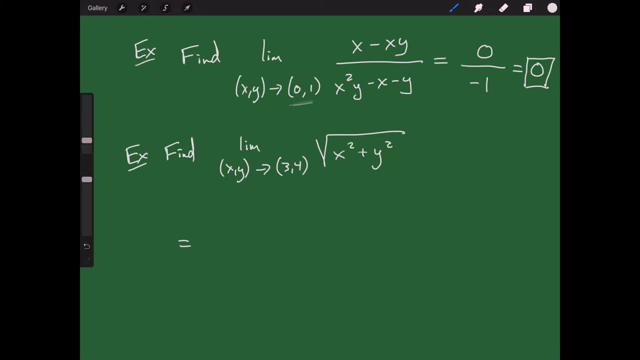 Again, if I can, let's just plug in the point. Am I going to cause division by 0 by plugging in 3, 4 for x and y? No, There's no division by 0 going to be happening, so I can just go ahead and plug it in and. 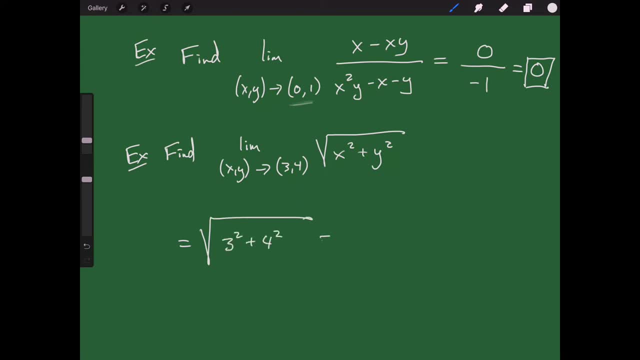 I get 3 squared plus 4 squared, which is the square root of 9, plus 16,, which is the square root of 25,, which is just 5.. Make sense. So the first thing that we would always do- and this we still do it now. 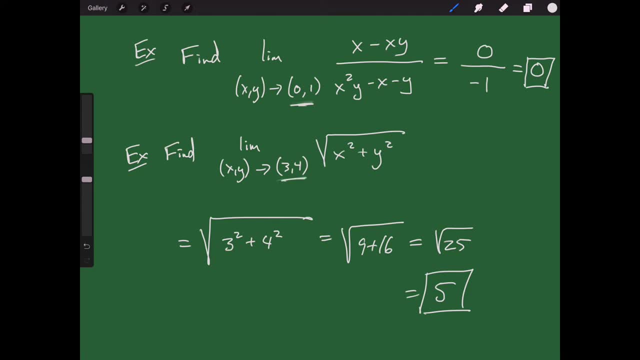 We just try to plug in the point itself. And if we can plug it in and we don't cause any division by 0, it's great. We can just get the limit that way. So we should probably look at an example where we do get some division by 0 and see what. 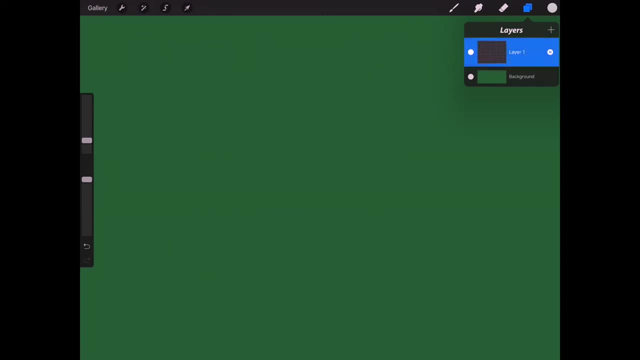 we do. Okay, So let's try this one. Let's take the limit as x y approaches 0.. Okay, So the limit approaches 0, 0 of x squared minus x y, divided by the square root of x minus the square root of y. 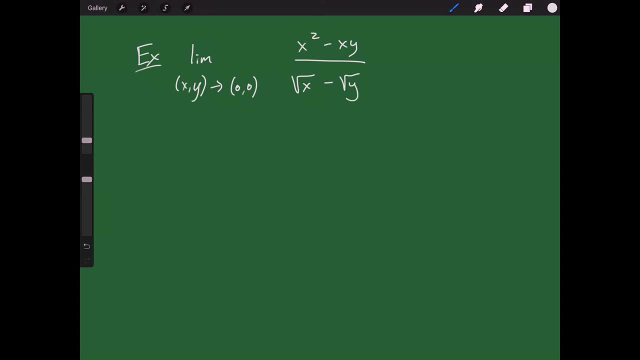 Okay. So now the first thing we might try is to plug in 0, 0. But if I plug in 0, 0, I get a 0 on the top and I get a 0 on the bottom, And that's not so good. 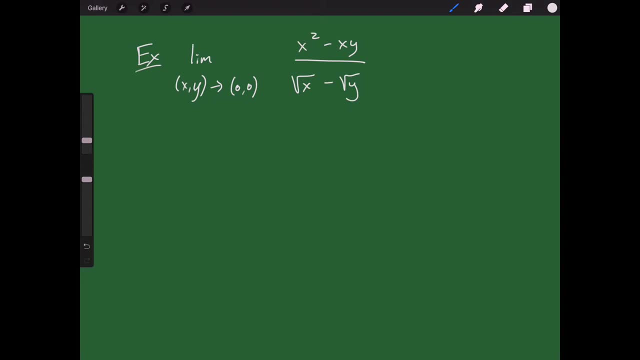 We know A limit is not typically going to give us 0 over 0. That's an indeterminate form. We don't like that. So the next question we typically ask is: can I factor this thing? Well, it doesn't look like I can factor the bottom, but I may be able to factor the top. 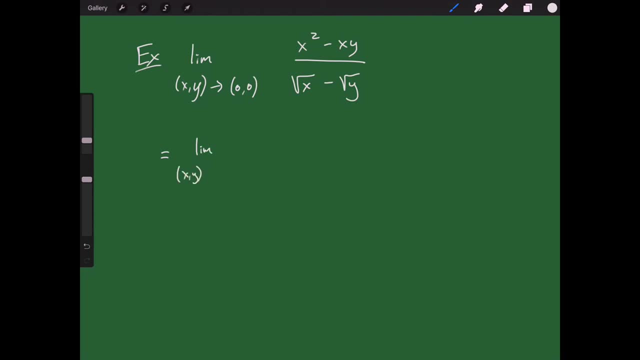 So I get the limit as x, y goes to 0, 0 of. On top I could factor out an x, And if I do, I get x times. Okay, So I get x times x minus y divided by the square root of x minus the square root of. 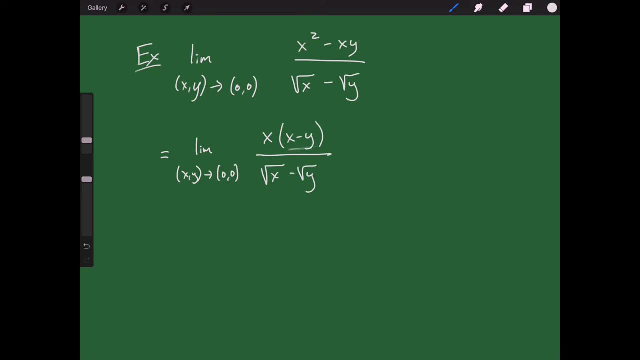 y, But x minus y up here. that's the difference of squares, if you think of x as the square root of x squared and y as the square root of y squared. So let's rewrite: This is the limit, as x, y goes to 0.. 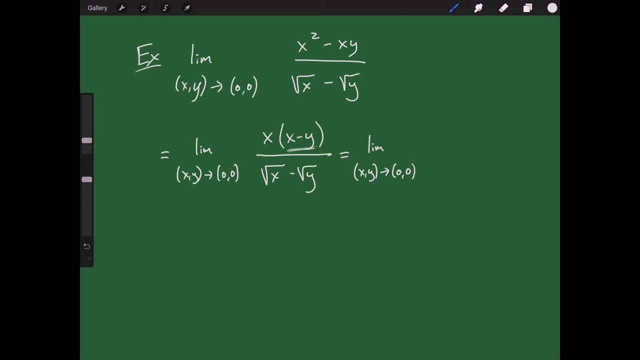 Okay, Okay, 0, 0 of x times square root of x minus square root y times the square root of x plus the square root of y divided by the square root of x minus the square root of y. So the square root of x minus the square root of y cancels on top and bottom and I'm left. 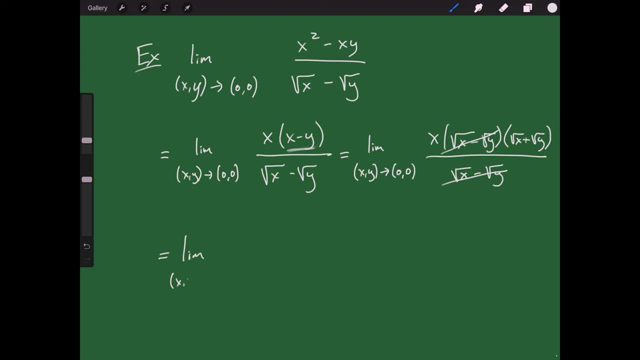 with the limit as x- y. Okay, So I get the limit as x- y goes to 0, 0 of x times square root of x plus the square root of y. And now the question is: can I just plug in 0s for x and y and not get division by 0 anymore? 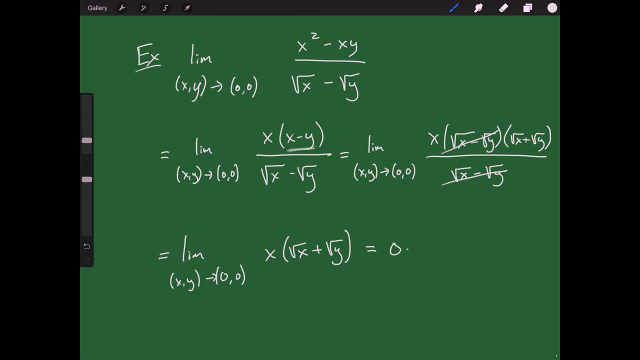 And the answer is yes, I can plug in 0s, and so I just get 0 times 0, which of course is 0. And so now all of the tricks that I know, So I can get division by a conjugate. 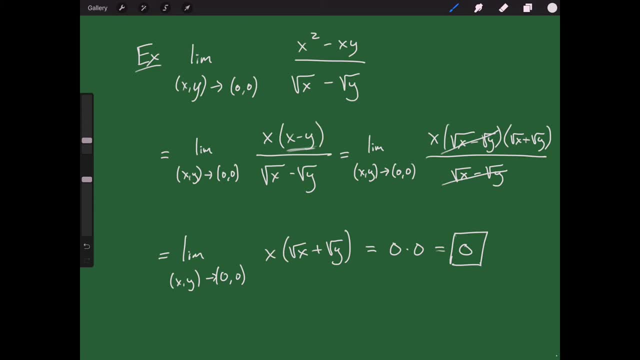 Okay, We can apply here and we can. potentially we can multiply the top and bottom by the same thing, Multiply by 1, combine fractions, all these different things that we've done before in two dimensions. We can now use the same tricks in three dimensions to find limits. 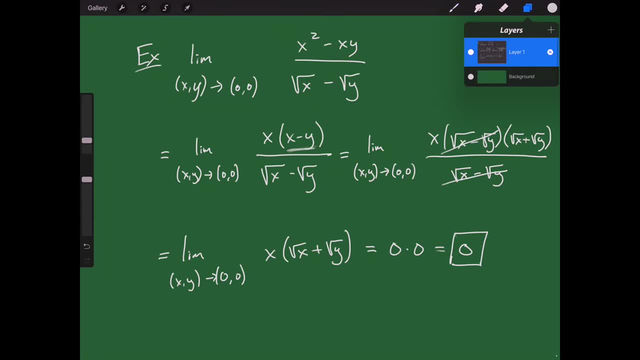 Okay. The second thing that I want to talk to you about now is, if we have limits in three dimensions, Can we find the limits in a number of numbers? Let's do it, Let's do it, Okay. dimensions. then we can also talk about continuity in three dimensions. so let's. 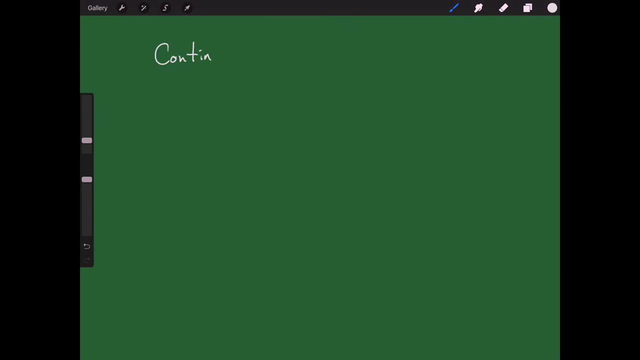 talk about continuity, and let's remind ourselves what continuity means. sometimes we think about continuity as I can draw something without picking up my pen. okay, that's kind of the simple way of thinking about it, but there's a better way to say it, and so let me write down the definition of continuity. 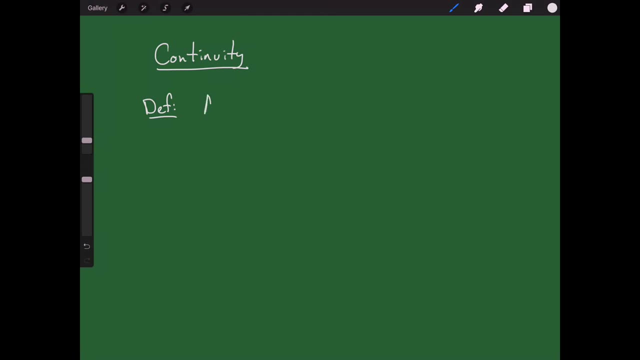 specifically in three dimensions. a function f of x? y is continuous at the point x sub 0, y sub 0, if a couple of things are true. first, f is defined at the point x, 0, y, 0 and 2. the limit, as x y goes to x, 0, y, 0 of f of x y exists. and three, those two values. 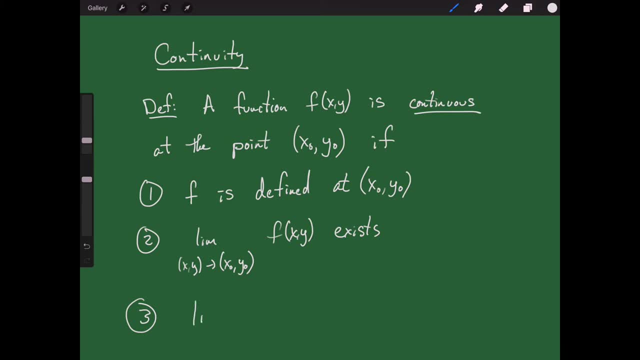 need to be the same. in other words, the limit, as x comma y goes to x 0 y 0 of f of x y needs to be the same as f of x 0 y 0. okay, if those three things. so we have a functional value, we have a limit value and those two values. 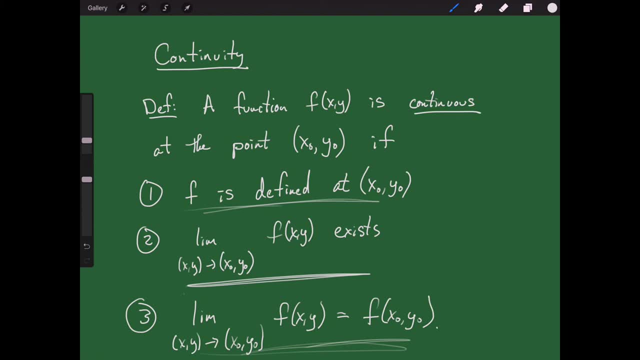 are the same thing, and that's what it means in two dimensions. to be a continuous function as well- is, you're defined at the point, you have a limit value at the point and the limit value equals the functional value. So no real change here. 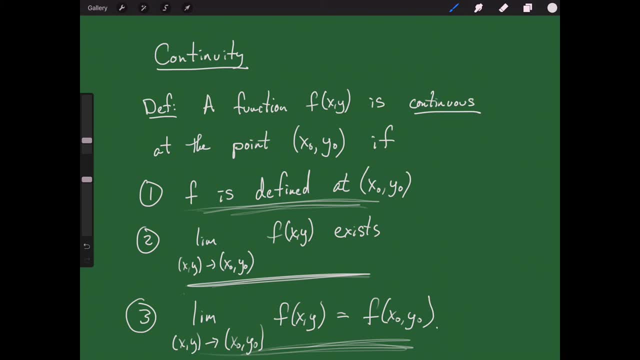 So another thing that we had in two dimensions, that we'll also define in three dimensions, is: what does it mean for a function to be continuous? This is continuous at a point, continuous at the point, But we can also talk about what does it mean for the entire function to be continuous. 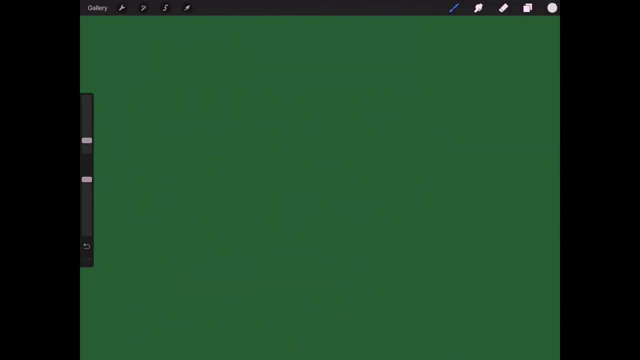 So let me write that definition down for you. So definition: a function is continuous if it is continuous at every point in its domain. Okay, so for the entire function to be continuous, then it needs to be continuous at every single point in its domain. 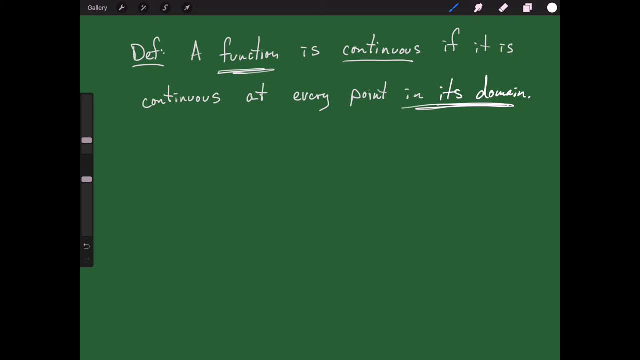 So it doesn't have to be continuous at points that aren't in its domain. It only has to be continuous at the points that are in the domain itself. Okay, Okay, So let's do a little example. So an example, Let's show. 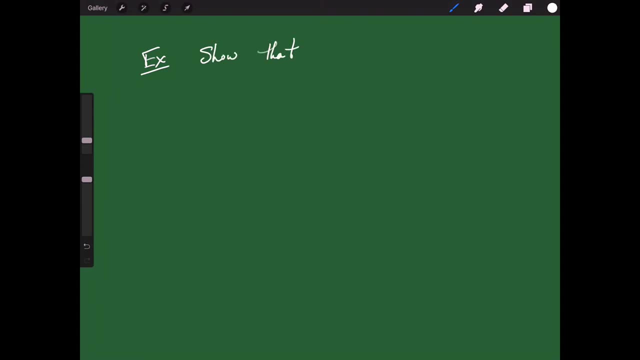 So the function f of x, y is equal to. it's going to be piecewise defined as 2xy divided by x squared plus y squared. If xy, if xy, if xy, if yx, if yx, if xy. 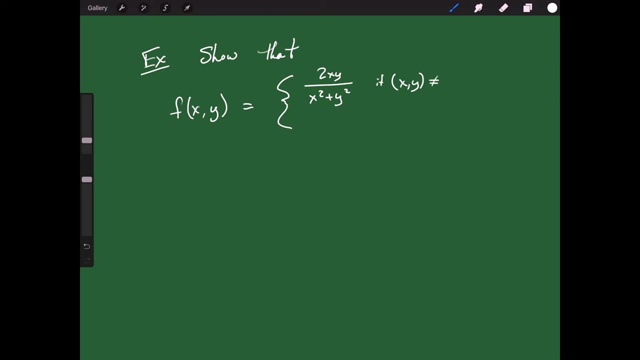 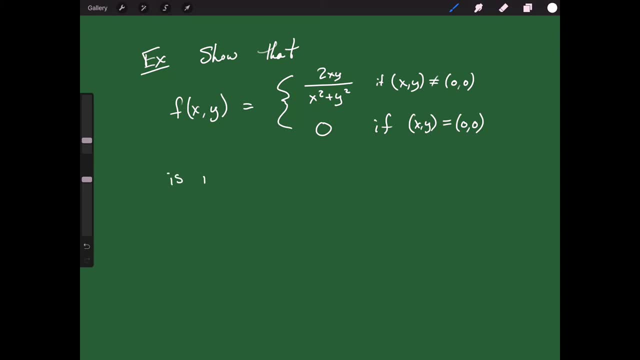 question, I guess, show that that is not continuous at the point zero, zero. all right. well, if you plug in zero zero to this function, you get zero. right, that's what the function says. you get zero. but the question is, are the points around that point zero, zero? are they close to zero, or could they be kind of far away? 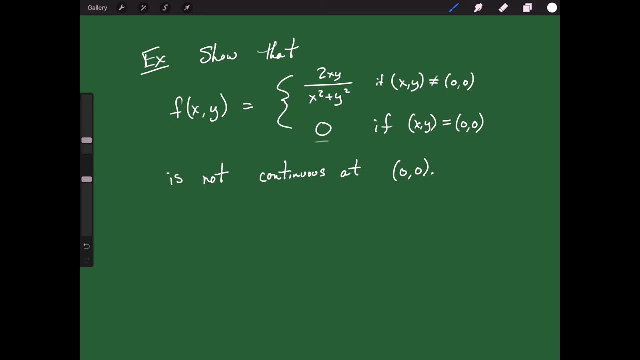 from zero. well, the thing is that if this thing is going to be continuous, then it needs really to be getting close to zero everywhere around it. so let's, how am I going to test everywhere around it when I'm really working in two dimensions in the XY plane? well, it's good enough for me to 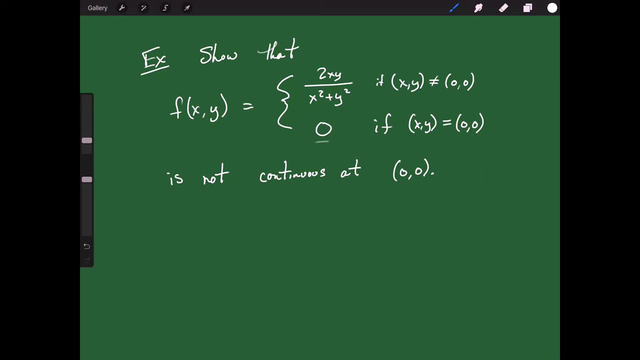 show that there are some places around it that are not getting close to zero. so what I'm going to do is I'm going to evaluate this function in the XY plane. so think of the XY plane for a second. here we are, XY plane, and I'm looking at 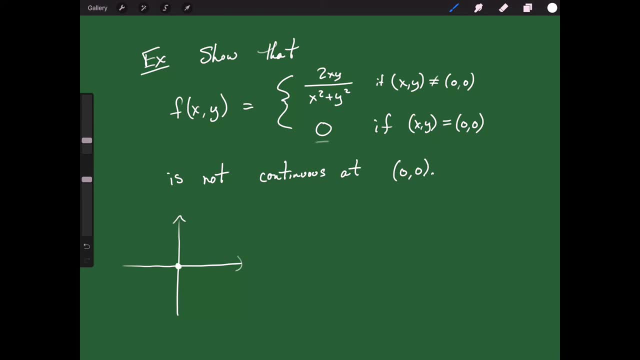 the point zero zero. I'm saying let's take some points that are close to zero zero and see if they're small. so what I'm going to do is let's look at just a little like neighborhood around zero zero and I want to take a specific path to zero zero and I'm going to call 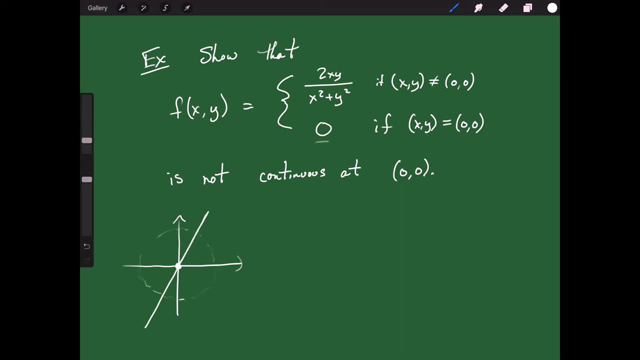 it a path that's along some line that goes through zero, zero. it could be any path. I'm just choosing a line path because it makes it easier for me, and then I'm going to say: well, what is that line? let's say that this line is y equal. 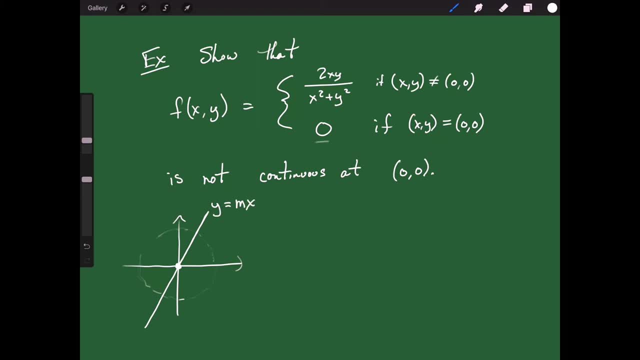 to mx. so what I'm going to do is I'm going to say, if I'm walking along this path and getting close to zero zero, then m is my functional value also getting close to zero. it should be, because I said, if things are close to zero, zero. 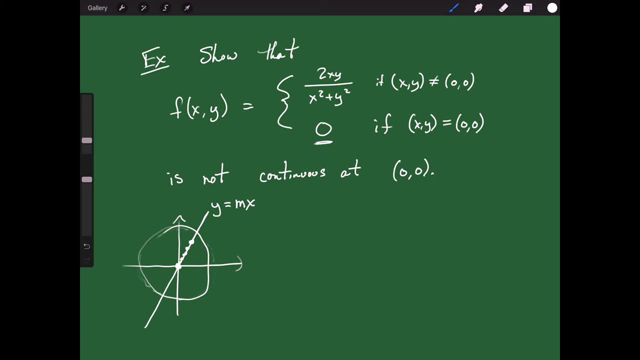 then their functional values should be close to zero. so what I want to do is I'm going to take this function f of XY and I'm going to evaluate it at Y is equal to this function MX. so in other words, let's replace the Y here with the MX. 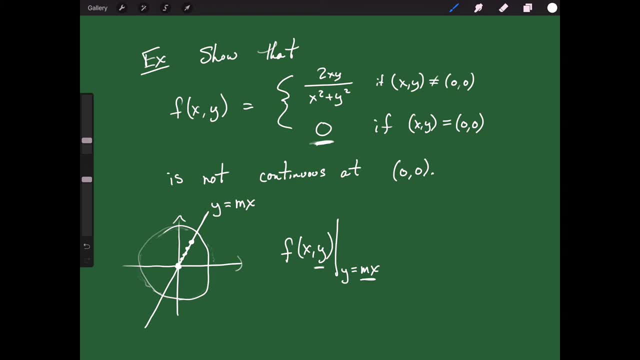 and see what happens. ok, so if I do that, let me rewrite here: I have F of XY and is equal to, evaluated at y equals MX, is equal to 2xy divided by x squared plus y squared, and that's going to be evaluated, or y equals MX. so now I'm just going to. 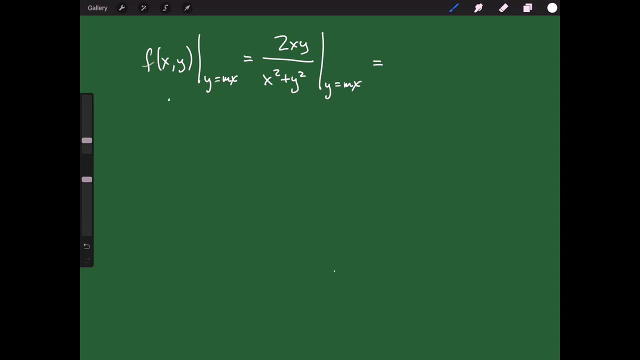 replace all my wives with MX's. so I get to X times Y. but why is MX divided by x squared plus y squared, but Y is MX squared. okay, let's rewrite that again. so I get this: is 2 M, x squared divided by. notice that, okay, the bottom is x squared plus m squared, x squared, so everything has an x squared. so i 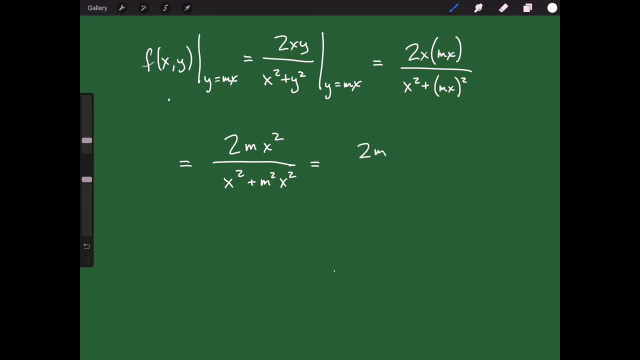 could cancel the x squared on top and bottom and i get a 2m on top and on bottom, i get 1 plus m squared. so this is interesting, right? uh, that what my value is, as i'm coming in towards zero, zero. well, it really really depends on the m, right? if m is one, what would i get out of this thing? 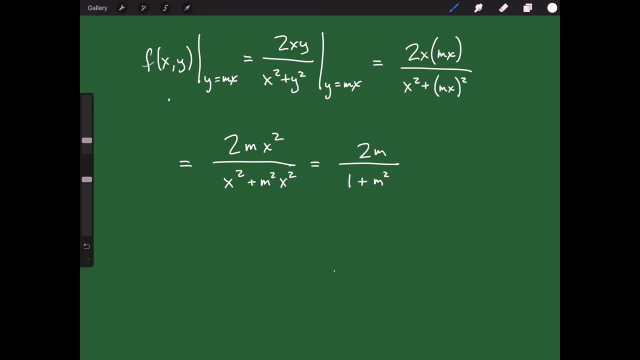 well, if m is one, the top would be two, the bottom would be two, i'd get one. now, is one close to zero? not really. it's kind of far away. it's not like point zero, zero, zero, one. it's one, a whole unit away. what if m were like two? then i'd get four over three. that's even. 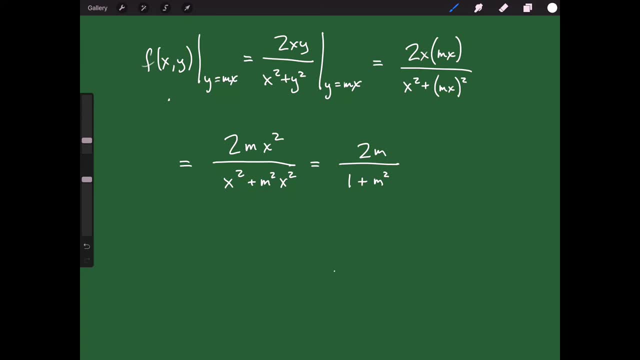 i'm sorry, if it were two, i'd get four over five. that's one. uh, it's a little closer than one was, but it's not very close to one. so what i'm seeing here is that this varies with my choice of m, so depending on what path i travel through the origin. 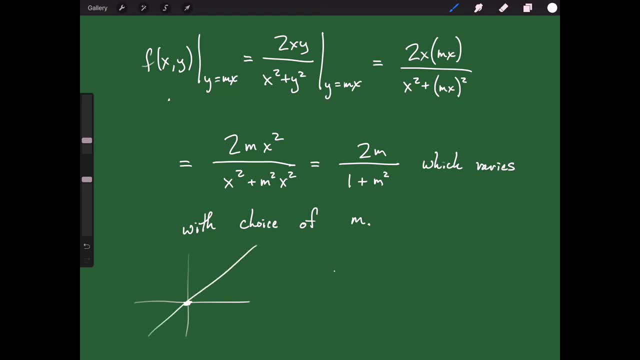 so if i take one line, i get one value. so this may be the one value that i'm going to get, and so here, m was one on the front. then a second line, one of these, so m will be m, and functions of this, or my value is: y equals x, and so m is one, and so the values. 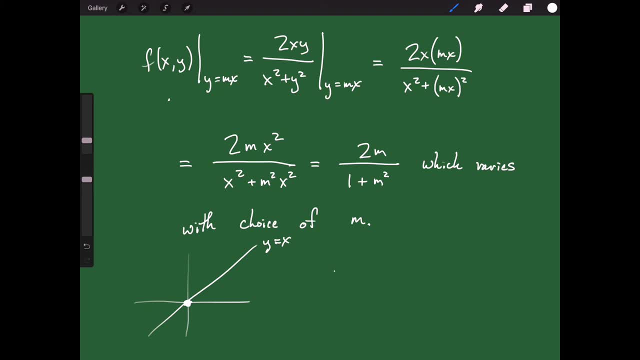 that are close to of this function are going to be one, but if i travel on a different path, like two, then the values of this function are going to be four-fifths. so what i'm seeing here is that it depends on what MA is line i'm going through, what value i get out of the m, which is the negative one, and on the x of the whatever mean. the negative being true, has an equation in addition to that: e Як. 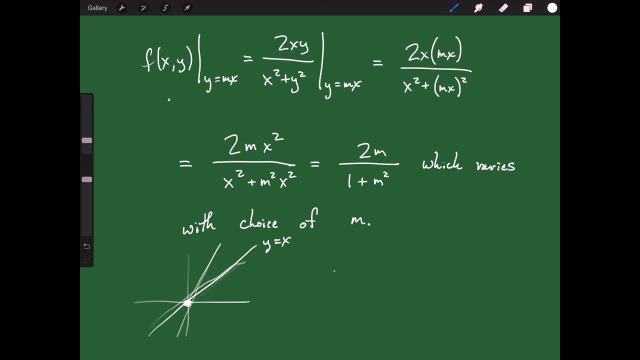 problem is one: what area of receive the right of the right of the factor? i know there has to be r will be k and the r have to be k plus k. if i leverage the loss out ofーー, on what line I'm going through? what value I get out of my function that when 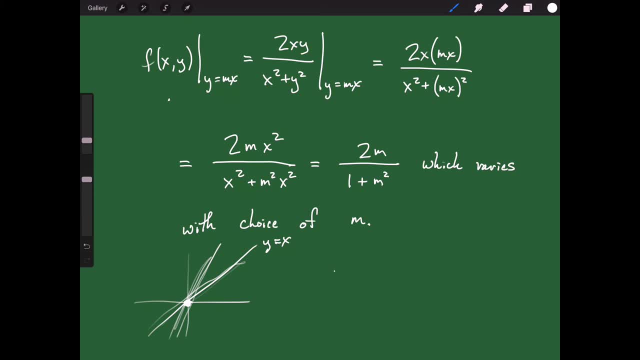 I'm close to the origin and they're not all the same. so this thing is not going to be continuous at 0, 0.. So the function is not continuous at 0, 0.. Functional values exist for all these points, but the functional values vary and as the functional values vary, 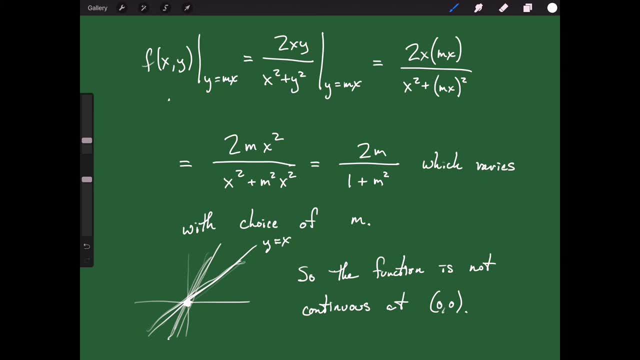 they vary very close to the origin as well, and so they're not getting close to zero, and that's basically what we needed. okay, so let's talk about what's called a two-path test. so a two-path test for non-existence of a limit. 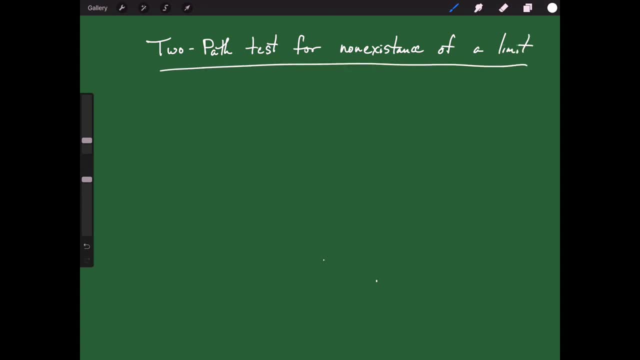 okay. so if a limit doesn't exist, how do you show that it doesn't exist? well, you really need to find two different paths on which you can approach that point and that have different um limits. and if it has two different limits in some sense, then it. 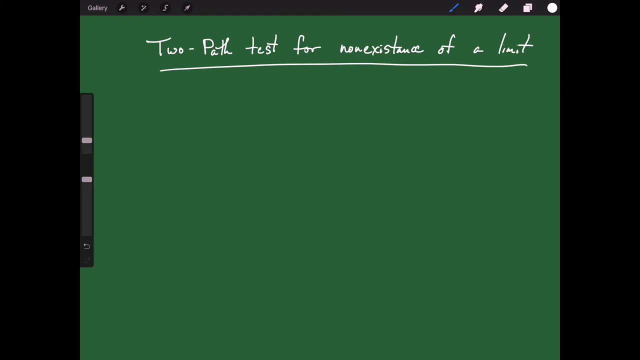 doesn't have a limit, because all the limits need to agree, no matter what path you're traveling. excuse me, had to sneeze, so let me write this down: if a function f of x- y has a different limit along two different paths, as x- y approaches. 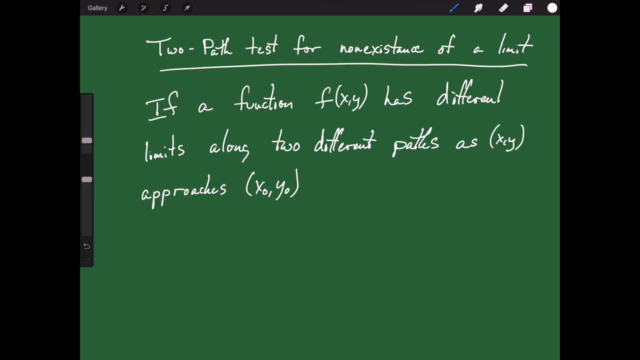 x 0, y 0, then the limit as x- y approaches x 0, y 0 of f, of x y to z, not exist. okay. so let me draw a picture of this just to show you. so let's say that i have a point in. 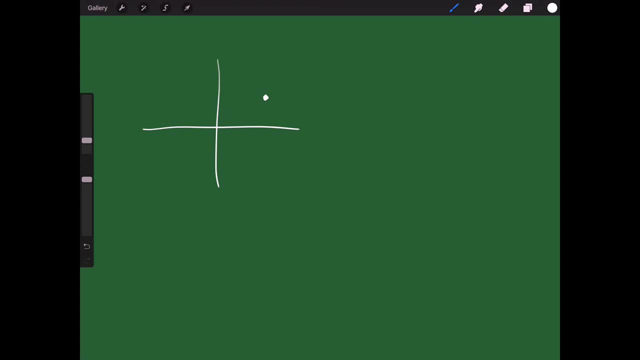 the x- y plane, it doesn't really matter. and i want to know what happens as we get close to x 0, y 0, okay, and i'm walking along one path and i say, as i'm getting close from dick this direction, my functional value is getting close to two, but as i walk at this point from this direction, 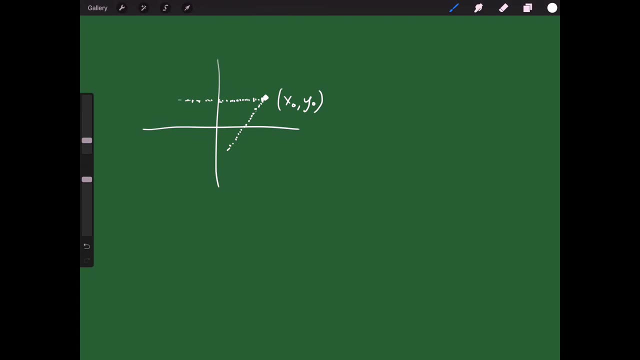 the functional values are getting close to three. well then, i'm getting close to. this path tells me the limit should be two. the other path tells me the limit should be three. well, it can't be both of those, so it must not have a limit. so if you can find two different pathways to the point 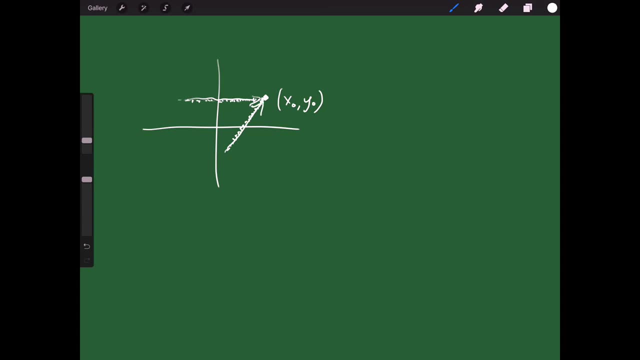 which tells you that the limit should be two different things. then what you find is it must not have a limit there at all. let's do an example of this so you can see kind of what what i mean. so a quick example: show that the function f of x, y. 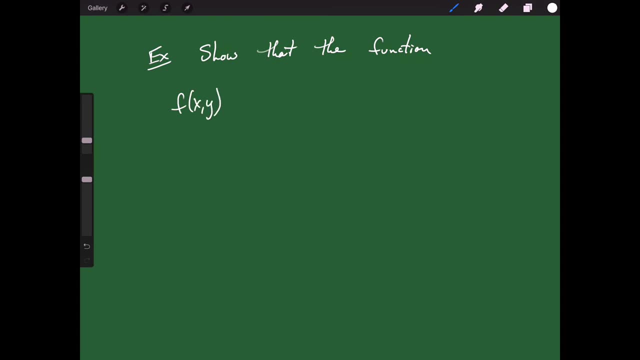 is equal to 2 x squared. y divided by x to the fourth, plus y squared, has no limit as x y approaches zero, zero. okay, so we have to choose what direction this thing walks along. so i can choose any path that goes through the origin. i just have to decide what path is going to be the most helpful to me. 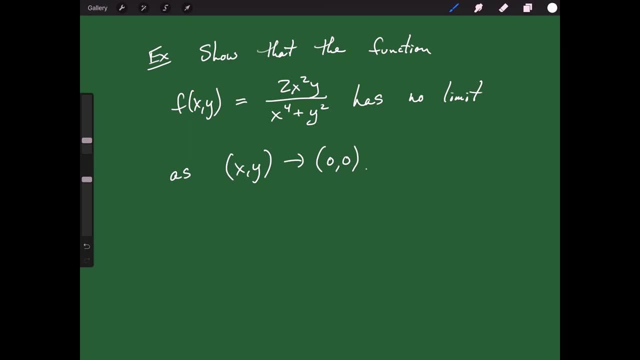 and what i see here is i've got some x squareds in my original function and i have some y's in my original function, so the path that's going to help me the most- that will make this thing simplify a little bit- is: i want to walk along the path. y equals some number k times x squared. now what is that path? 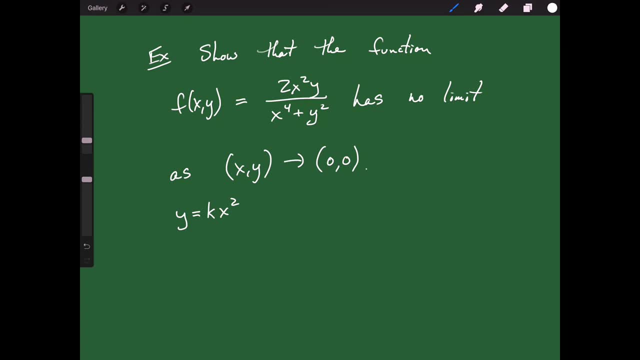 that is a parabolic path that goes through the origin. but i don't know what k is. so here's the origin and like, let's say that k is this path. k was equal to one, then I'm walking along the path of just my standard parabola. If k was. 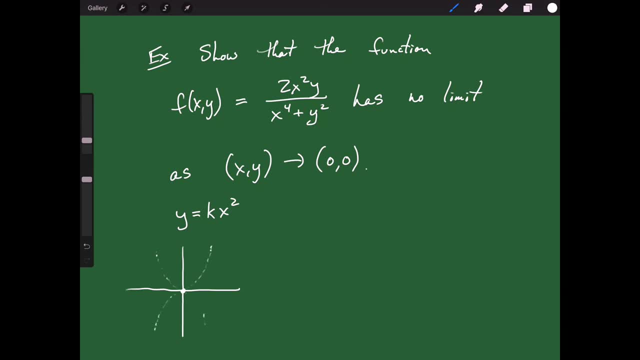 negative one, then I'm walking along the path of that parabola flipped. If k is equal to two or something, then I have kind of a stretched parabola that I'm walking along. So it just depends on what I choose for k. So in essence I'm doing a lot of paths at the same time, walking along all these. 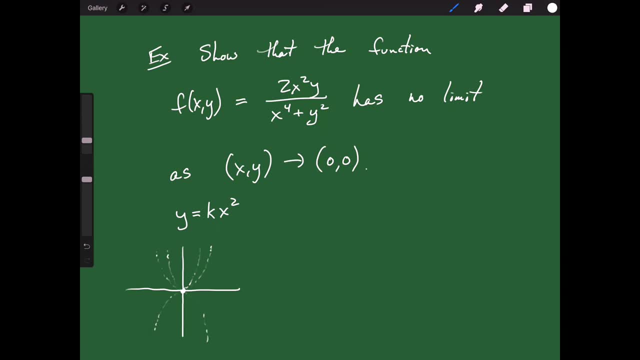 various parabolic paths. And you might ask: well, why did you pick a parabola and not a line? Just because the parabola is going to make things simplify better, You could use a line, But if it doesn't simplify, the line may not help you very much. Okay, so what I want to do is I want 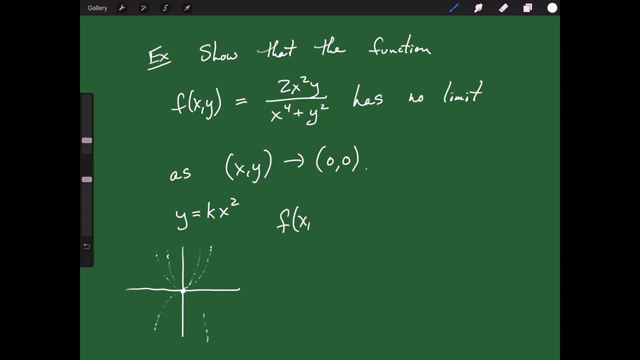 to look at this function f of x- y evaluated where y is kx squared, And definitely your path, though, needs to go through the point that you're evaluating, And it does in this case. Okay, so if I want to evaluate that function where y is equal to kx squared, then I get 2x squared times y. 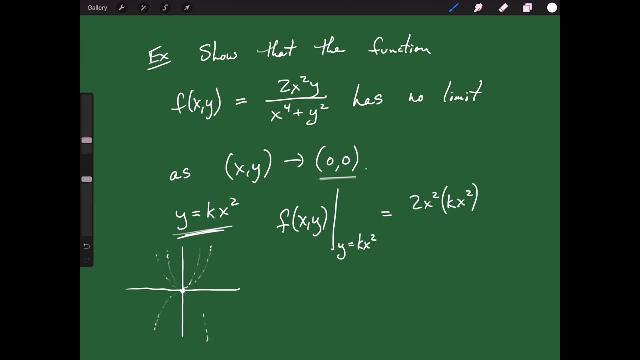 but y now is kx squared divided by x to the fourth, plus y squared or kx squared squared. Okay, we can simplify that a little bit more And on top I would just get 2k times x to the fourth. 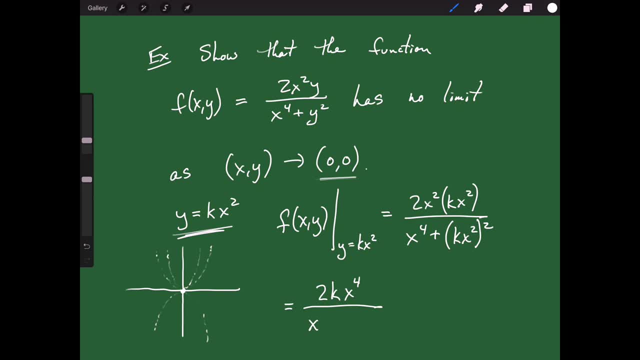 And on the bottom I would get x to the fourth plus k squared x to the fourth. So all of the x to the fourths cancel and I get 2k divided by 1 plus k squared. And now the question is: so it's saying that if I take the path, kx squared. 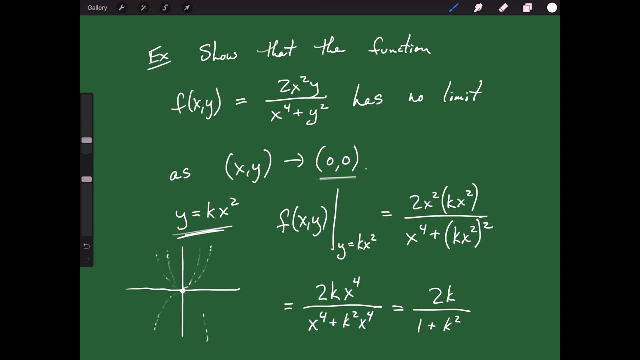 this is what I'm going to get out of the function. Okay, Now what if k was 1?? If k was 1,, what am I going to get out as all of the functional values here? Well, if k is 1, then I'll get out as my functional values. 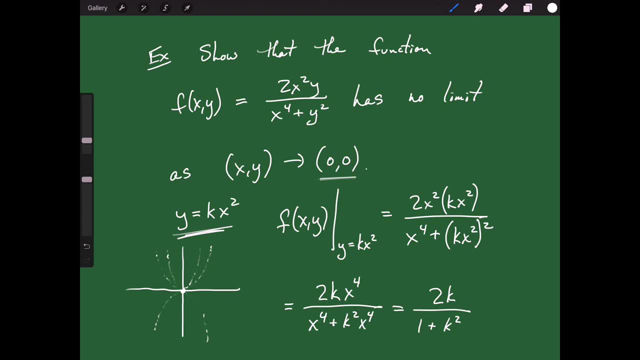 2 over 2,, which is 1.. Okay, so what I'm seeing is, if I take the path where- if k is 1, then what I'm doing is I'm saying, okay, let's walk along this parabola to go to 0.. So, as I get, 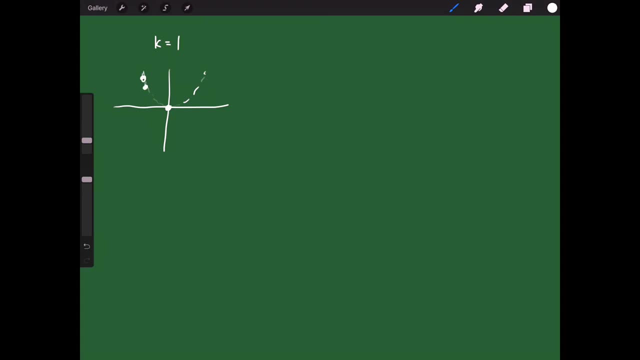 close to this point 0,. what are all of these functional values? Well, I said, if k is 1, then I just get 2k over 1 plus k squared. If k is 1, this is 2 over 2, which is 1.. Okay so, if I'm walking along this,